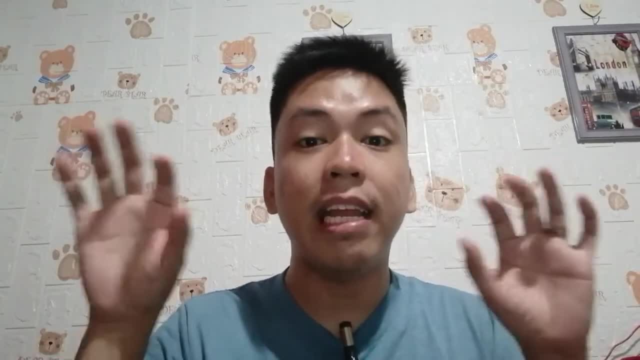 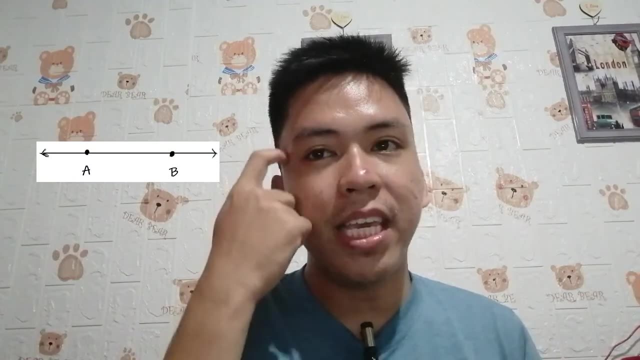 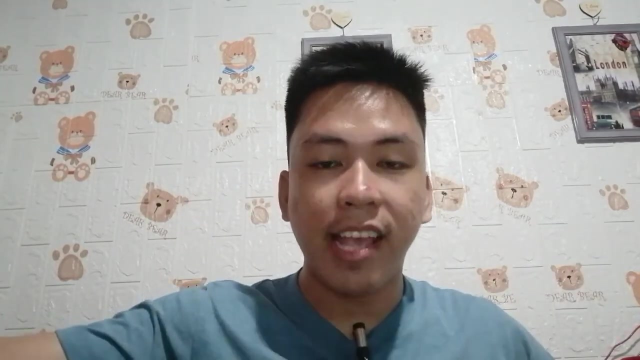 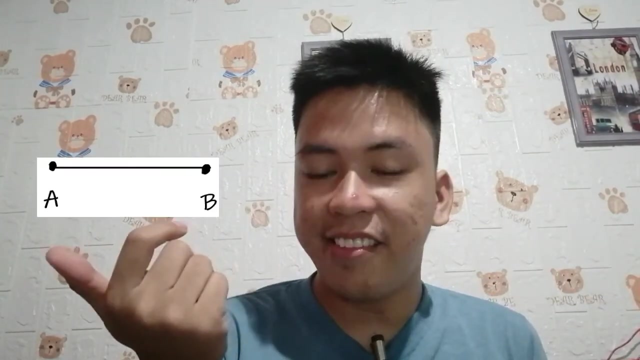 connecting from one point to the other point, as present in the line. when we say line, denoted by the symbol, that would be a representation of a straight line connecting from point A to B and extended to forever side-by-side. that's it. so, just to make sure this is a definition, I mean the symbol for a line. 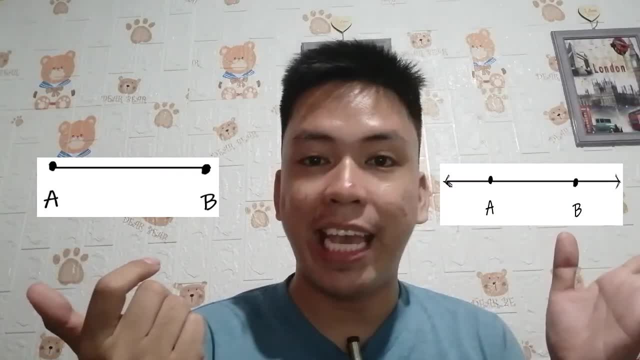 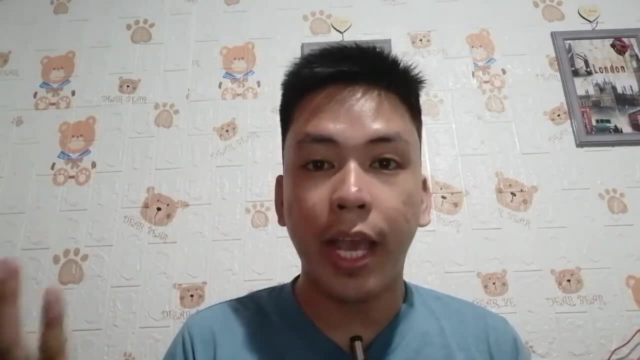 segment and this is for the symbol for the line. now, when we are studying with plane geometry, mostly we are only dealing with the line segment. why? because we are only focusing on the finite length of a certain object, and we are only focusing on the finite length of a certain object. 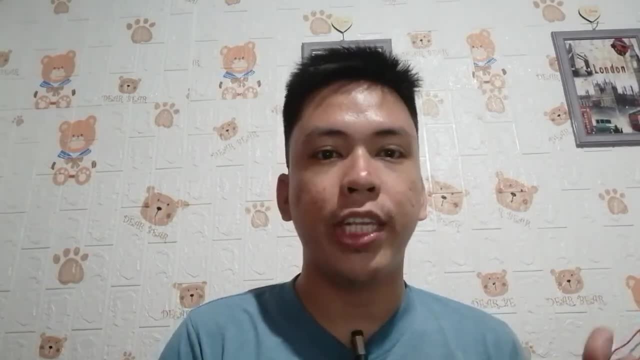 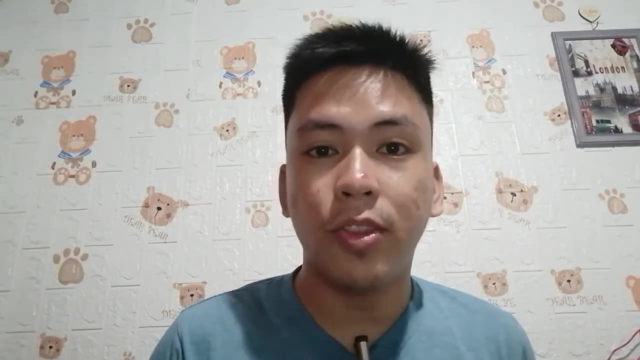 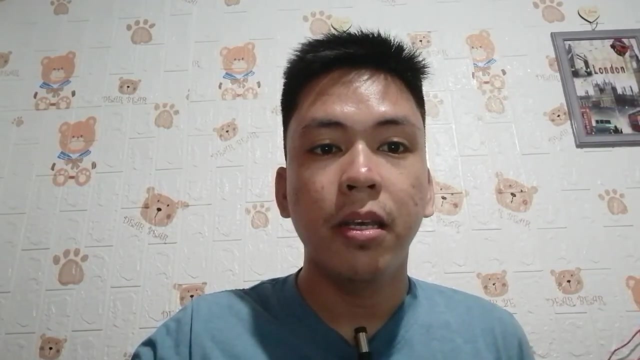 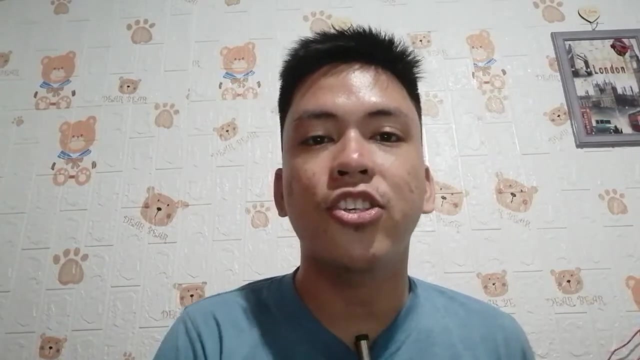 the reason why we are introducing with a concept of points, line and line segments is that we are actually upgrading as days go by. when we study with a plane geometry, we are concerned with the study of representations of objects because to make sure that we have understood on the right page. 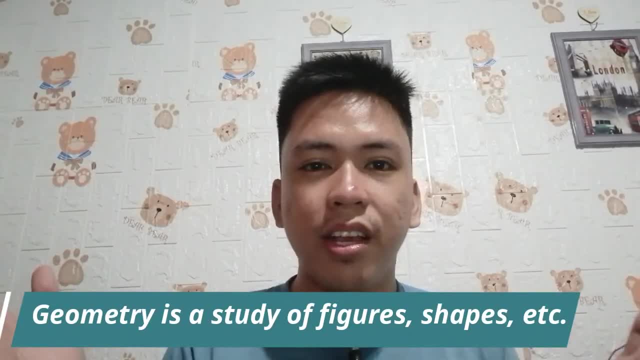 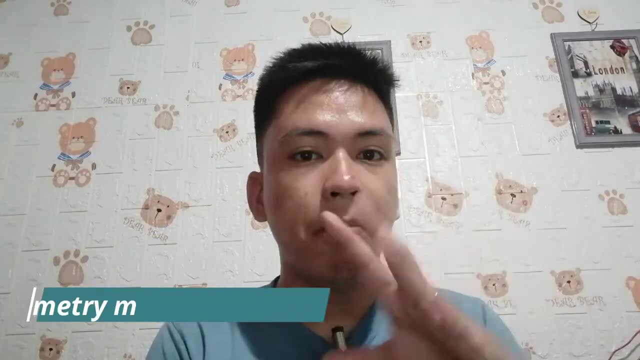 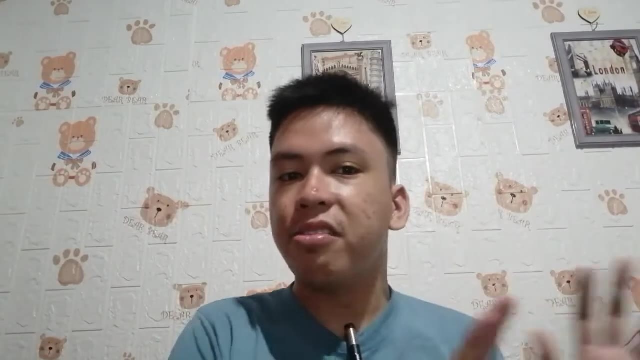 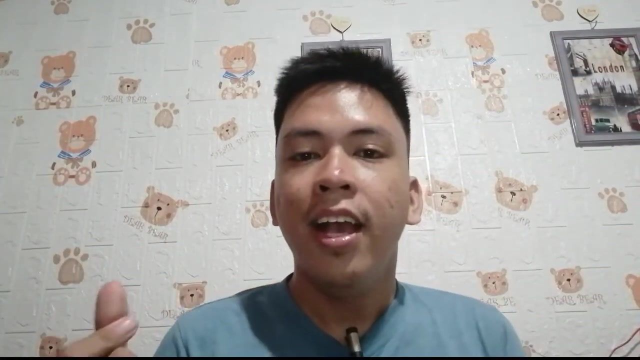 a geometry is the study of shapes, lines, figures that are present in earth. by the way, geo means earth, met. three means uh from the latin word um, measurement. so that's it. but we're not really concerned with that history and so on with the geometry. we are concerned with the fundamental tool, tools present in geometry. now, um. 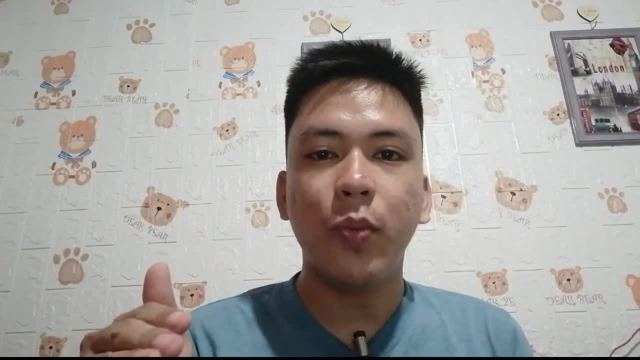 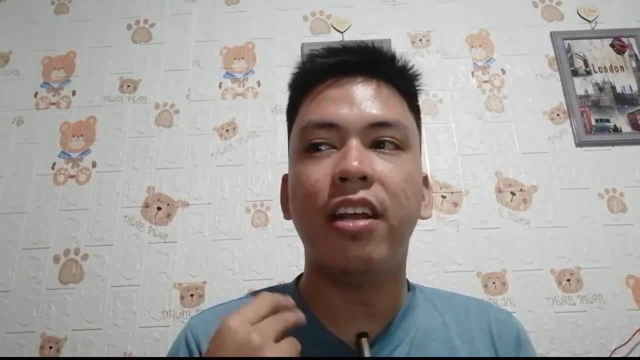 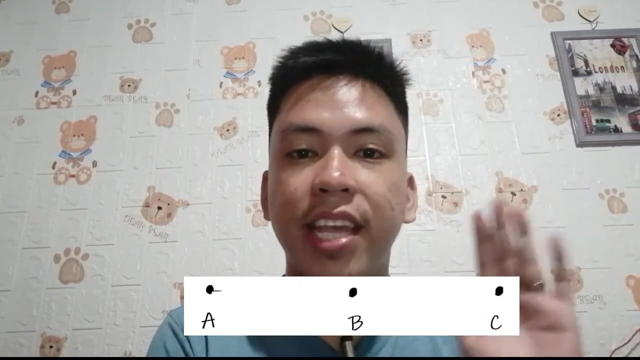 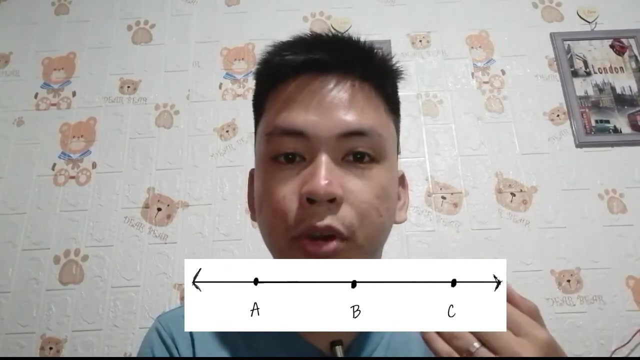 um, now that we know already what a line and a line segment is, consider we have three locations, so with, let's say, three points: a, b and c. now, in this case you have a, b and c and assuming that a, b and c lies on the same line, so that means there is a straight line connecting to the three. 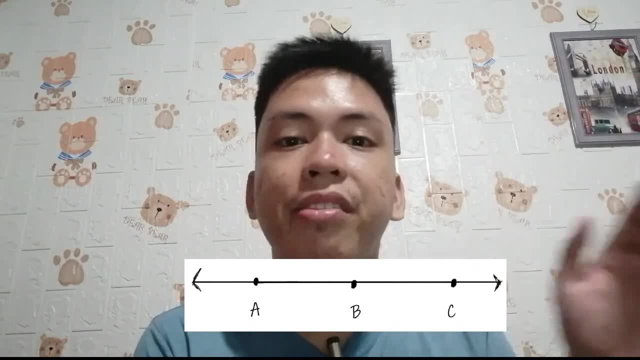 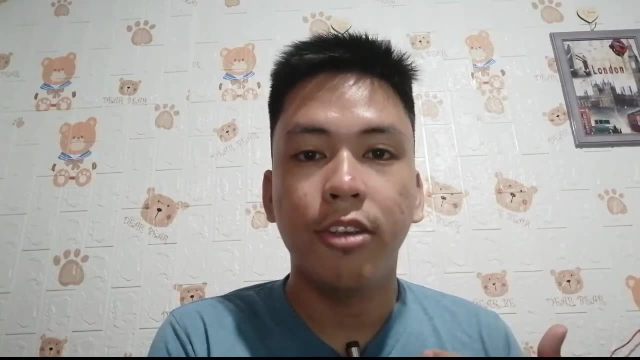 points. so if those three points are present on the straight line, we would have a line segment that lies on the same line. so that means there is a straight line. we would say that those three points are collinear. so they are collinear to each other. that's it. 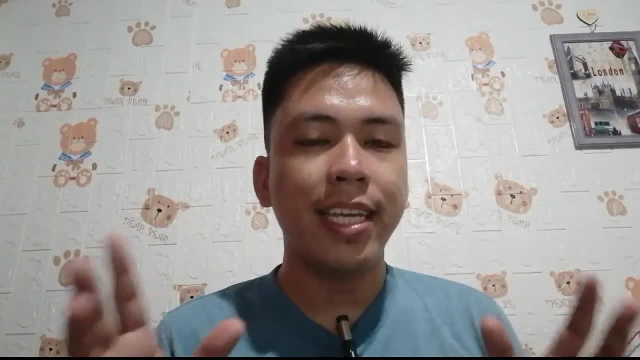 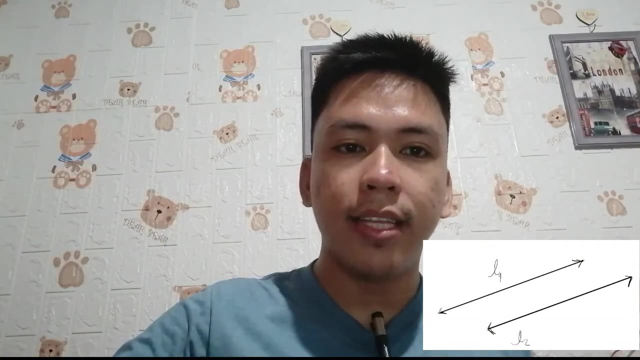 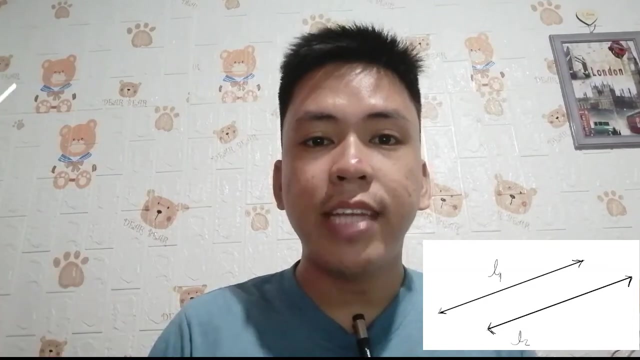 okay, so, um, now that we know what a line is, say, for example, we're given two lines. so, assuming that you would extend that tool forever side by side in such a way that the lines never meet with each other, so that means those are parallel lines. so if you would like to examine a certain point on a 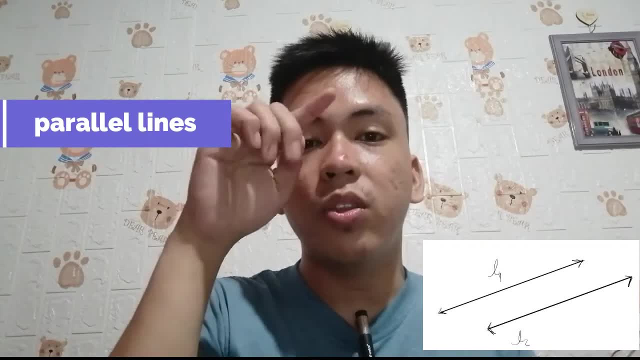 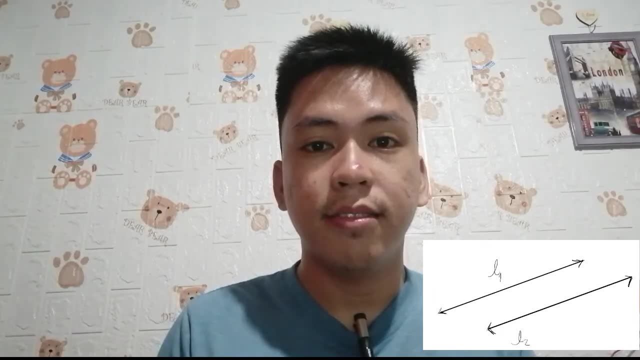 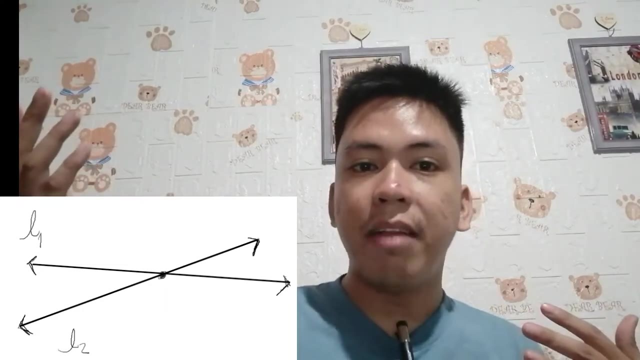 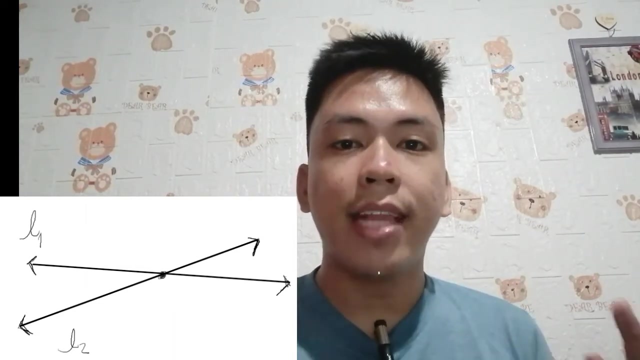 first line, and then you would say that those three points are collinear to each other. that's it now suppose, for example, that if you have two lines again and you would extend that side by side until the such extension would result that the two lines would intersect at a certain point, then that two 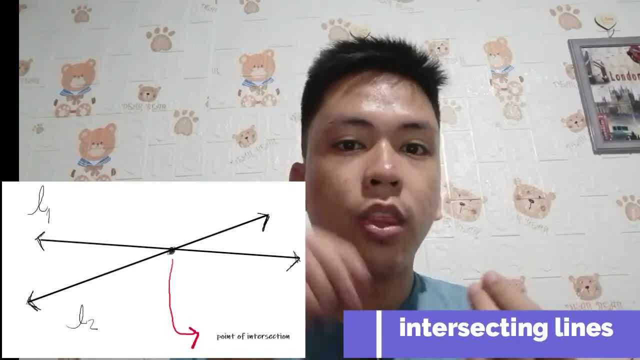 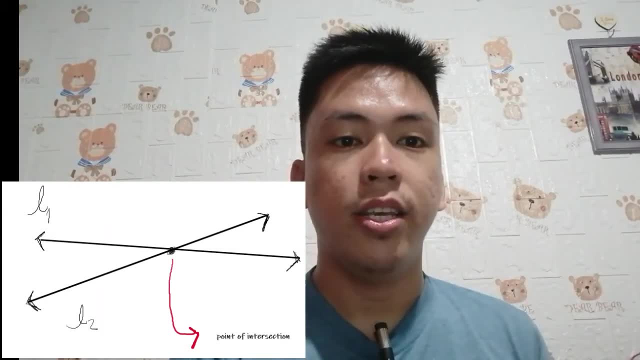 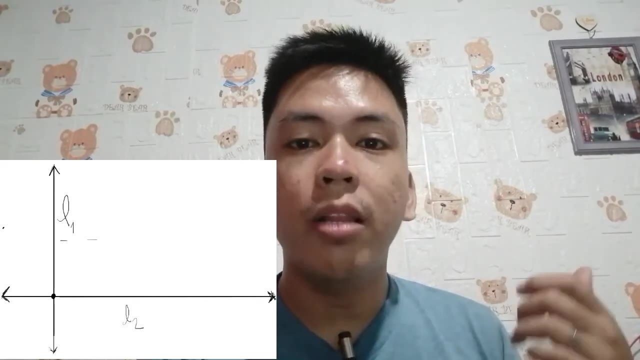 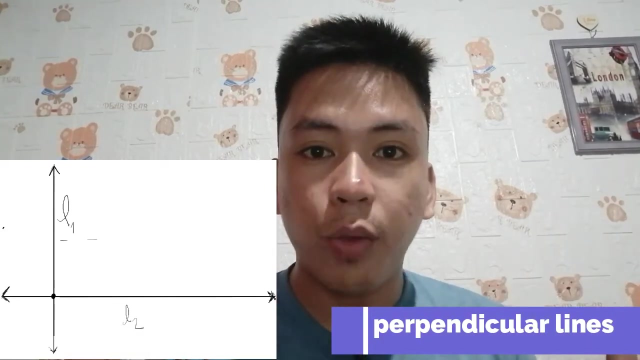 lines would actually intersecting lines. the point at which two lines intersect at a certain point intersect is the point of intersection. and one special type of intersecting lines is what we call perpendicular lines. so this is a special type of intersecting lines at which, when these lines intersect with each other, they form like. 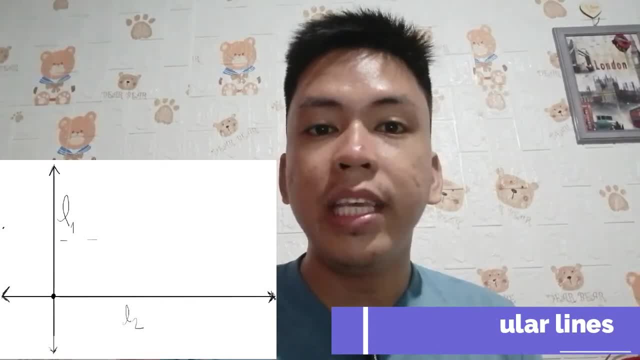 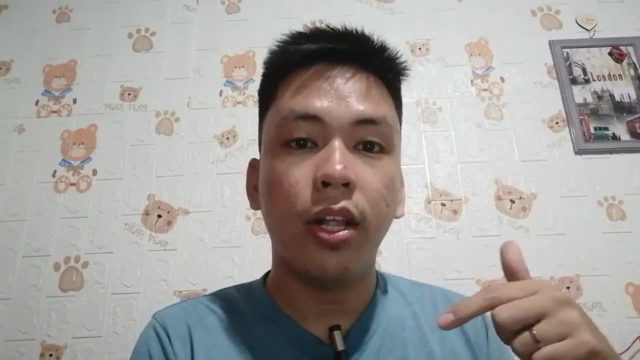 a square corner. so when we deal that with the high um, the further topics in plane geometry or in trigonometry, we would say that the two lines intersect at a certain point and that's it. we call that as a right angle. they are forming right angle, 90 degrees, so they have a projection. 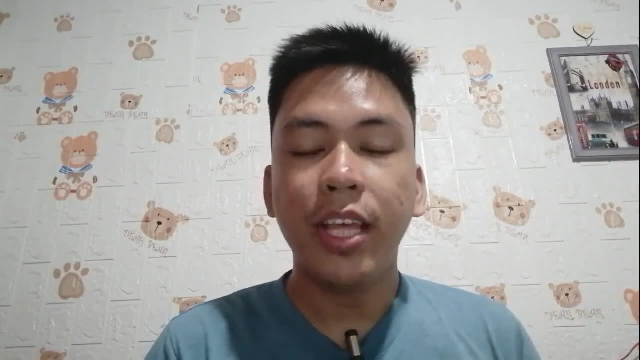 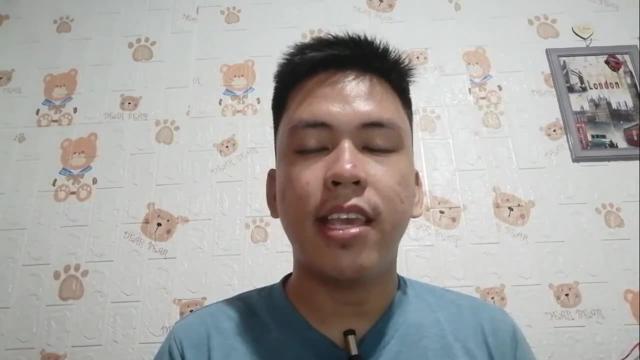 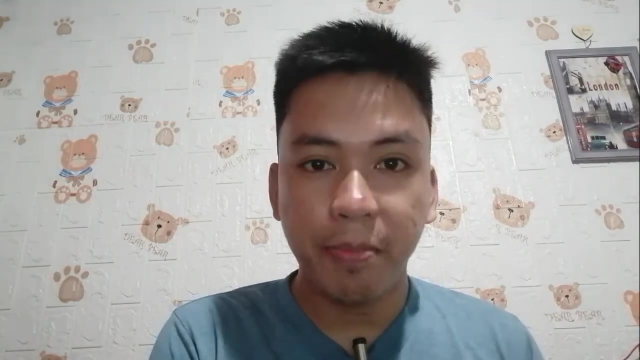 90 degrees to each other. now that we've known what a point, a line, a line, segment and intersecting lines- uh, perpendicular lines and parallel lines are, then, um, those are actually a concept of what two-dimensional spaces are. so, in this case, um, we will introduce the concept of what a two-dimensional 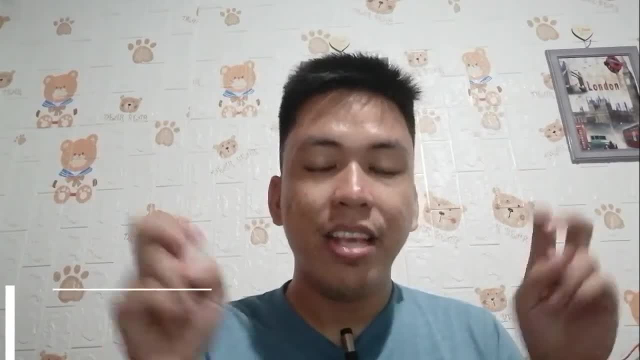 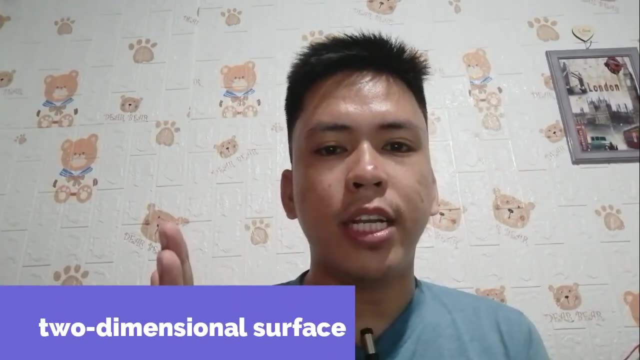 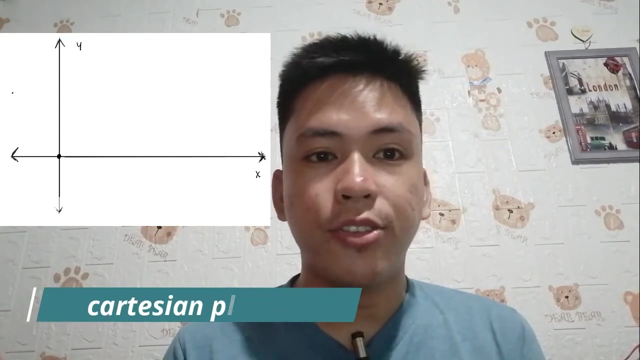 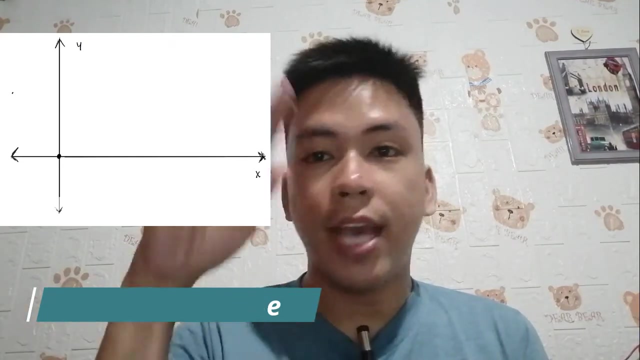 plane is because a plane is a flat two-dimensional space, so it's a two-dimensional surface. so this is actually, um, um say, for example, uh, the cartesian plane. so that is actually a two-dimensional space wherein you can move your points, uh, from going to the right or to the left, or to the up, or 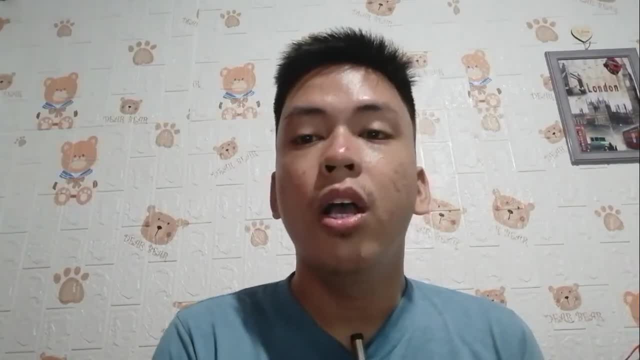 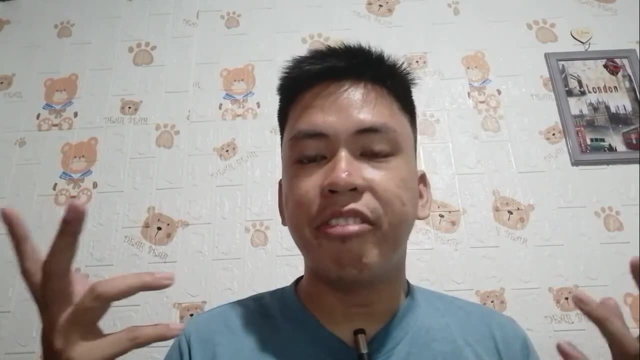 to the down. so that is actually a representations of whip that we place on the plane, and then we can think of a plane in a two-dimensional space. so that is actually a two-dimensional map and, um, we see that, you see in the upper right-hand corner of the graph that there is a plane just like an. 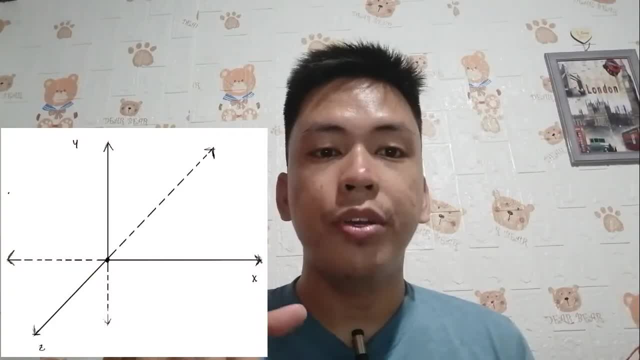 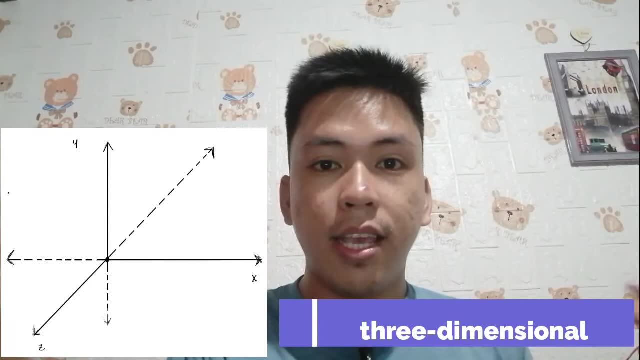 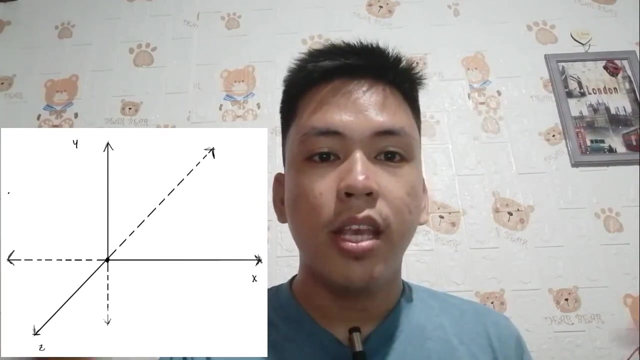 object here that we can draw here in geometry. but in the event that we're in um, aside from just um, representing a plane wherein you can move right or left or up and down, whether you can extract outside from the plane or inside on the plane, that's a three-dimensional plane and that way, if 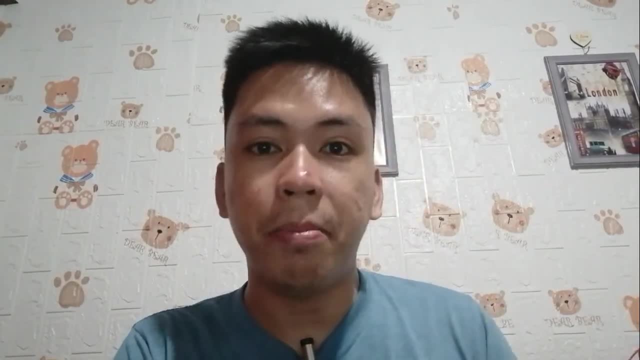 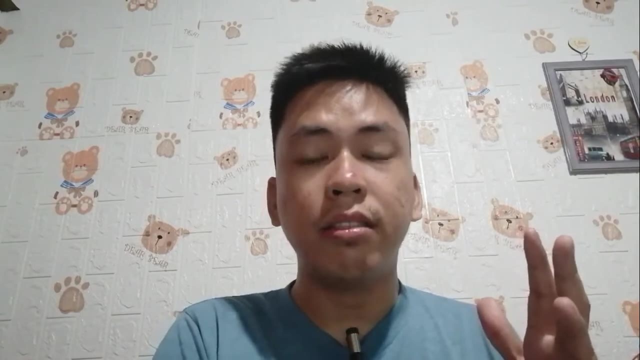 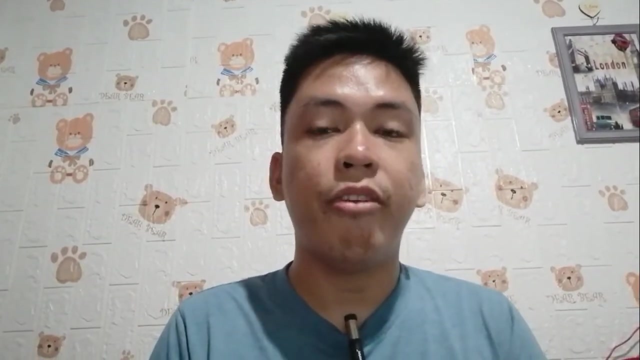 dimensional spaces, then we're talking a very complicated type of a plane which is way beyond humans way of solving. so in in the concept of mathematics we are dealing with a three-dimensional case and we generalize in order for us to understand further um and dimensional space. so 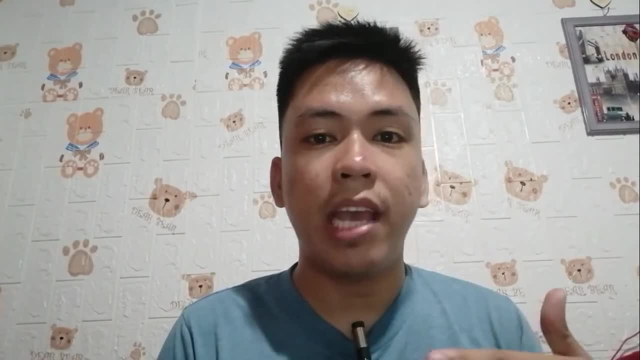 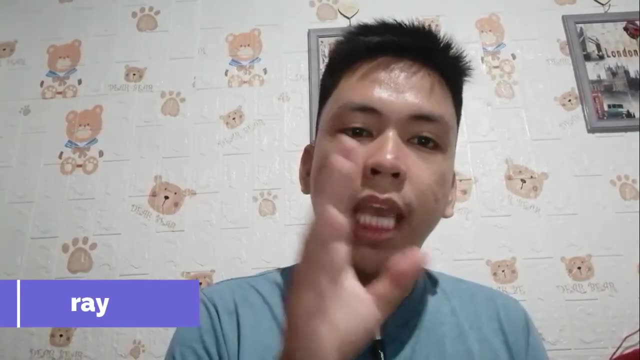 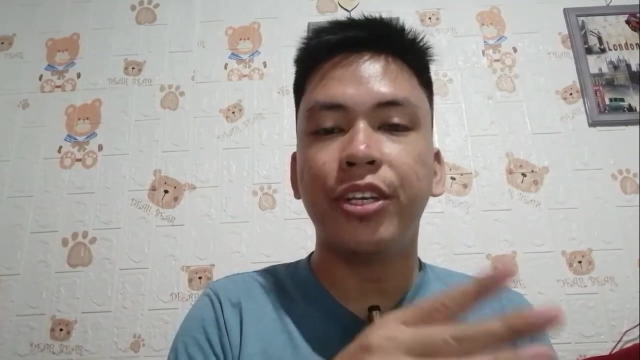 here um for the concept of geometry as an introduction to trigonometry. we will um start with introducing what array is. so remember that we have um two points that will determine lines and line segment. now suppose, for example, if you're given again a point a so and another point b. 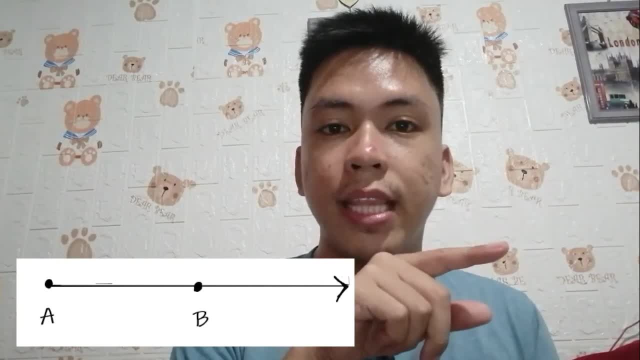 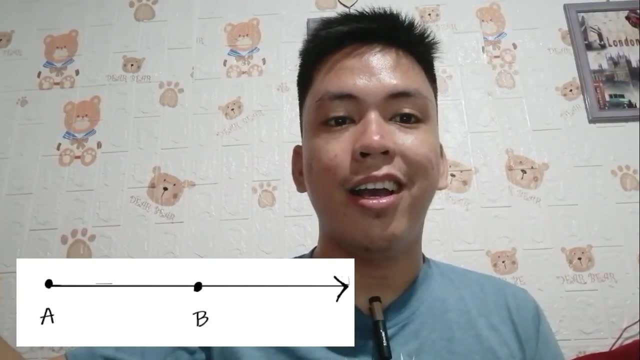 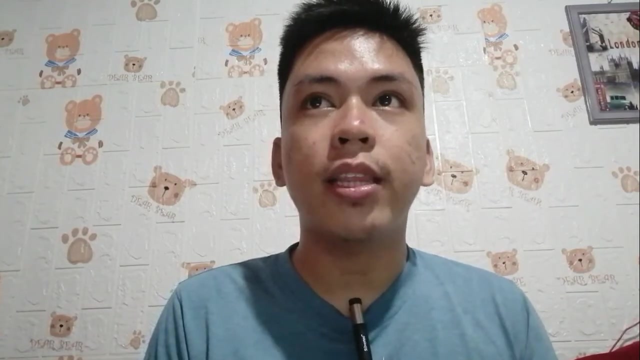 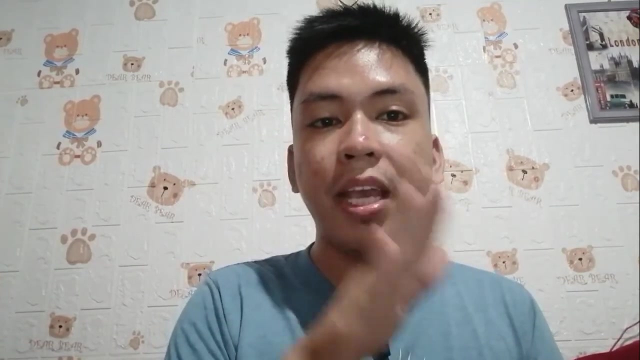 and starting from the point a, there, um, you would create a line, a straight line connecting from a to b, and extend it to forever. that would be array. but take note of the difference because, um earlier we have defined what a line segment is. a line segment is a straight, um, a straight line connecting from a to b. 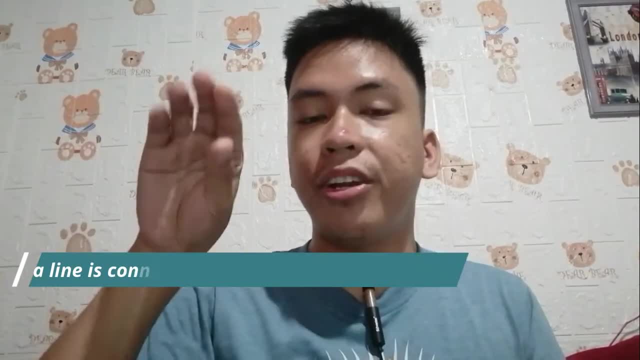 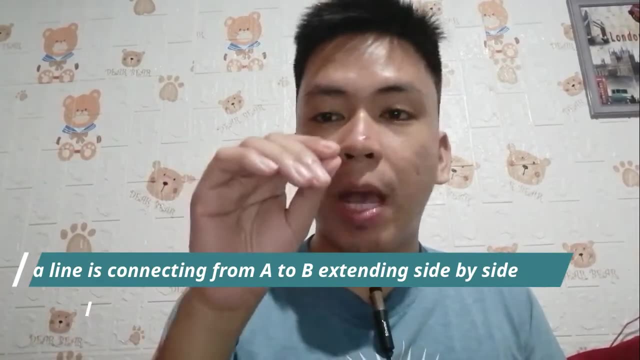 and connect and extend it to forever side by side. so that means starting from b, it extends to forever and starting from a extends to forever. that's a line, but a portion of it, wherein you start from a, you don't. you don't have to extend it. 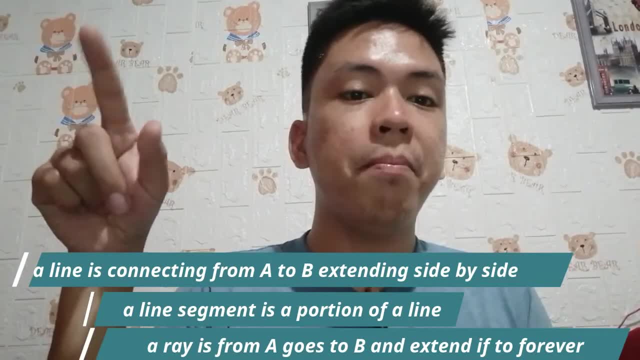 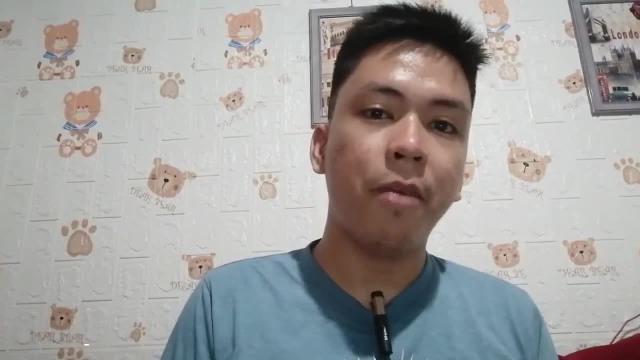 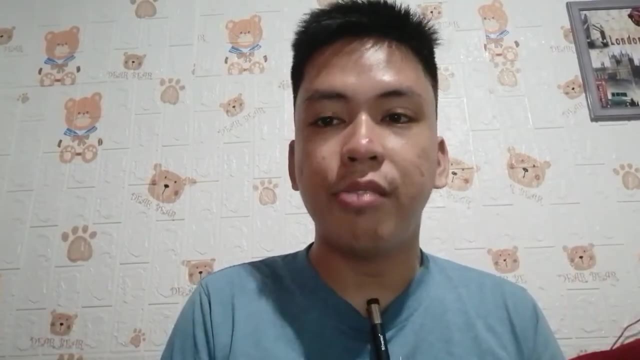 from the left of a, but starting from a goes to b and b goes to forever, then that's array. okay, now array will actually form an angle if you have two rays, at which, um, the starting point of two rays is the same point. so say, for example, you have points, 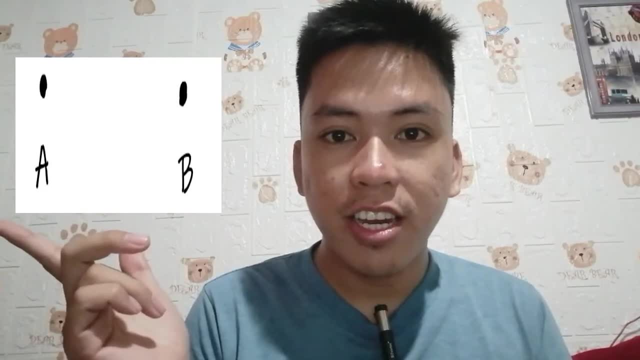 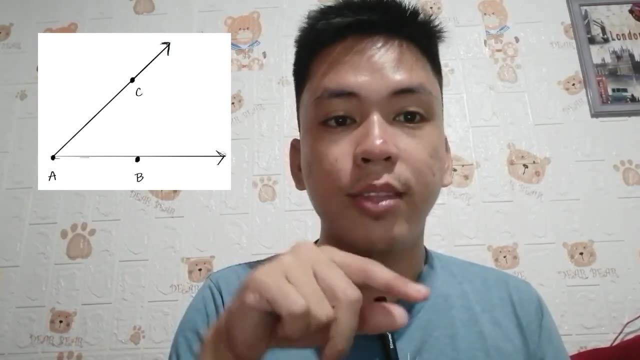 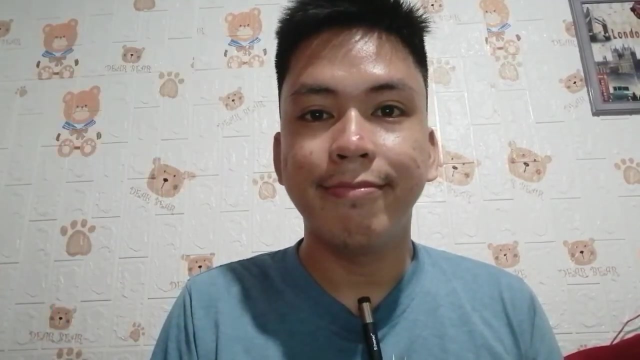 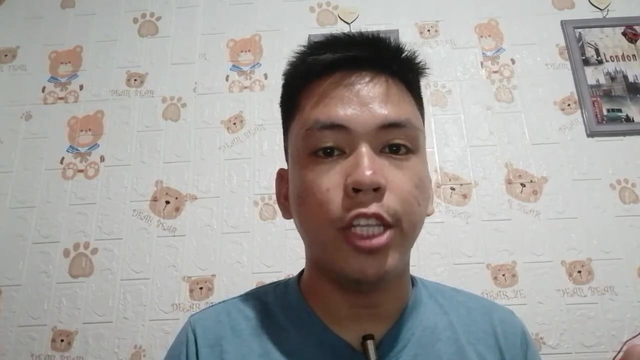 a, b and c, as given by this figure. now, um, if suppose, for example, you would have a ray starting from a to b and starting from a to c, and extend it to forever because it's a ray, then that would form an angle. that's it now. speaking of the angle, we have different types of angle at 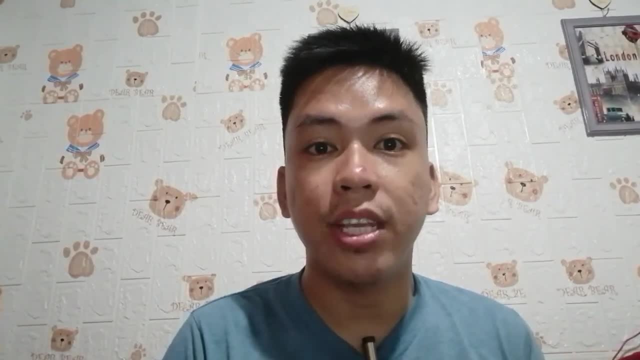 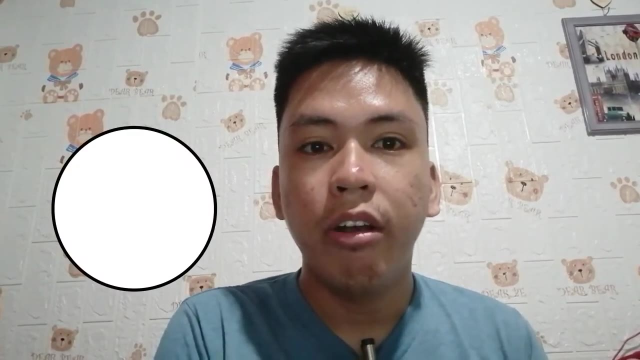 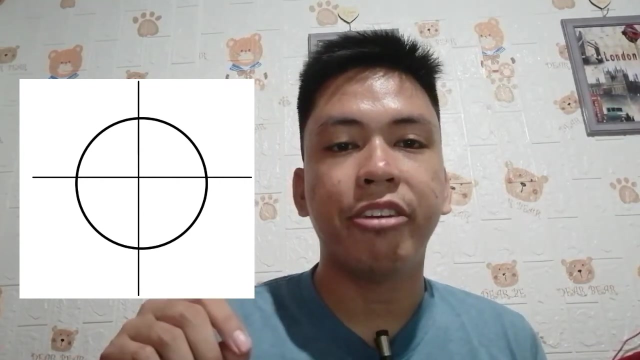 which they differ from their certain measurement, so they are based on a circle. so suppose a circle is divided into four, part at which, um, they are divided by means of having a perpendicular line and a perpendicular line. so say, for example, you have perpendicular lines, so that means they form a square corner. 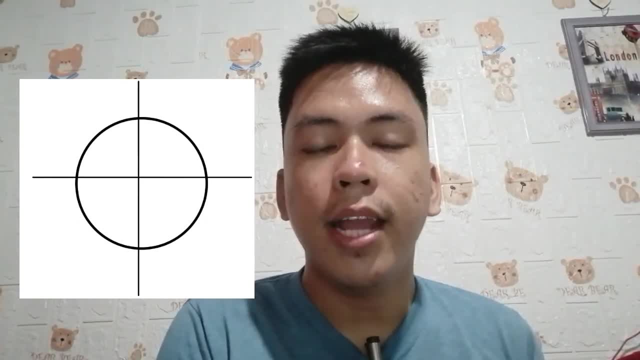 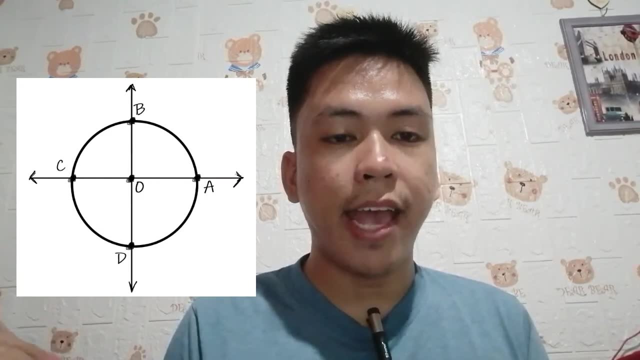 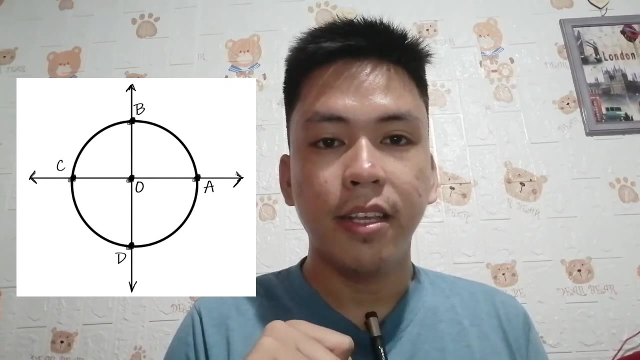 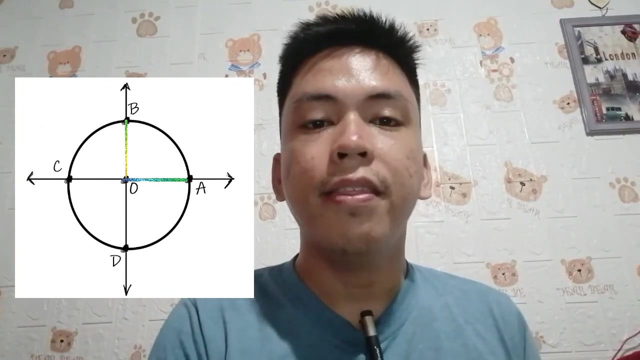 on the intersection point. so let us consider um two lines here at which you'd have the race as um zero a, zero b, zero c and zero d. so let's consider, for example, zero a to zero b, so that means the race zero a and zero b, that two rays form 90 degrees. 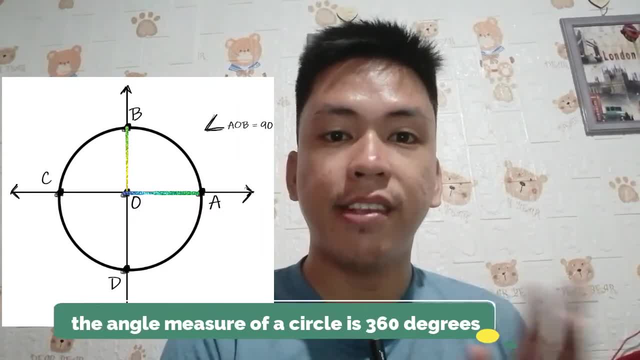 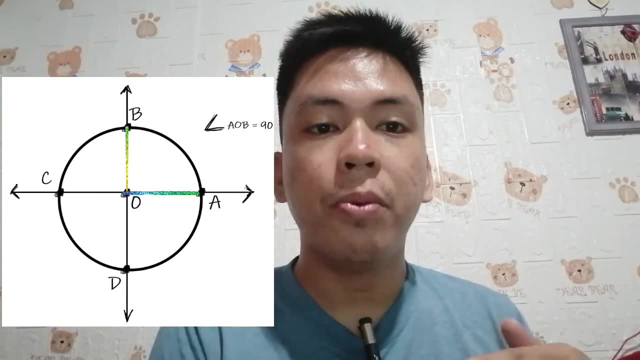 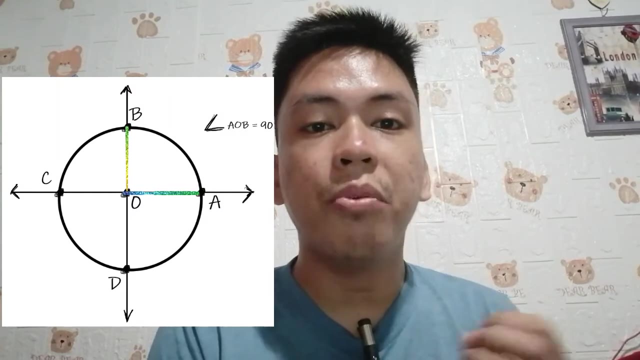 why? because an a circle is measured 360. so that means if you divide it by four, they are 90 degrees with each other. so the race zero b and zero c form 90 degrees and zero c to zero d forms 90 degrees, same with the race zero a to zero d. okay, 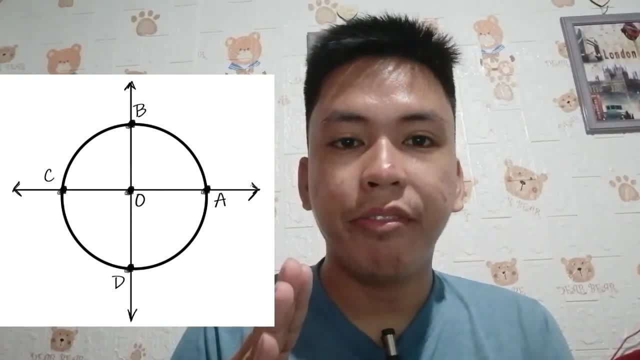 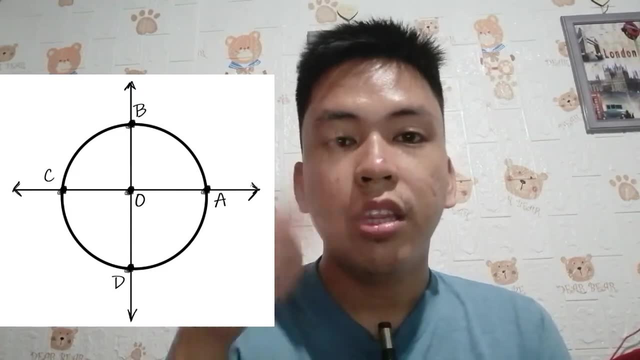 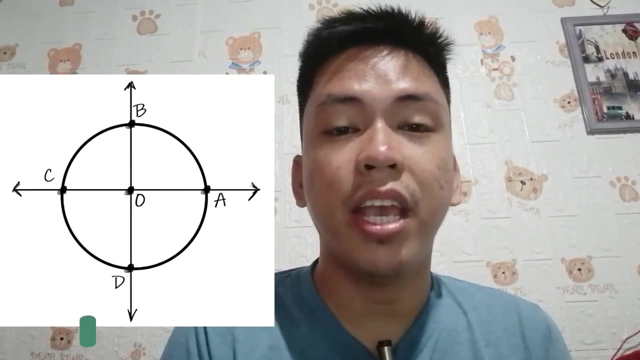 so that is the basis there. so if remember that, um, two rays can form an angle, so which means the four division of a circle is already an angle, and in that case if they form 90 degrees with each other, then they are so-called right angle. if suppose, for example, you would have a 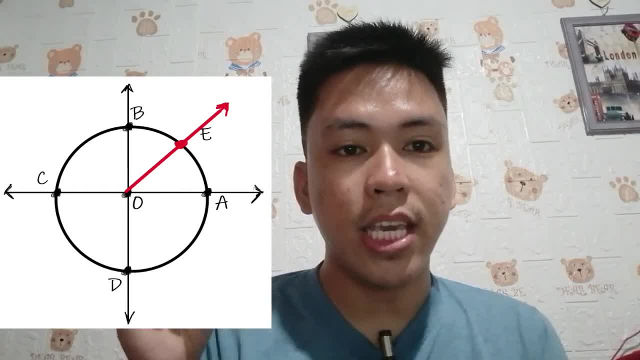 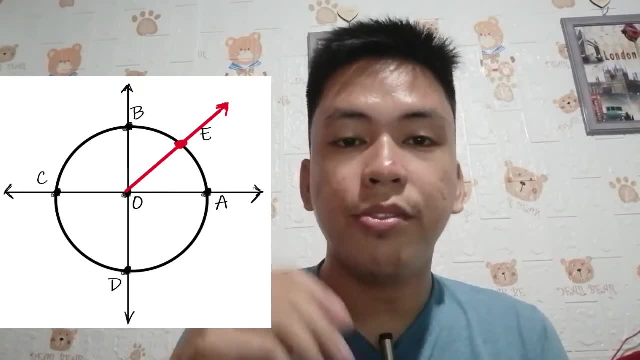 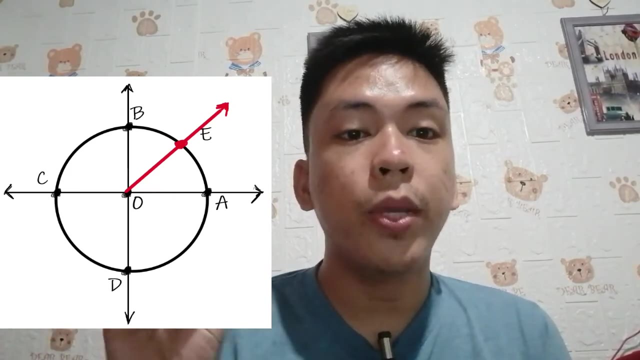 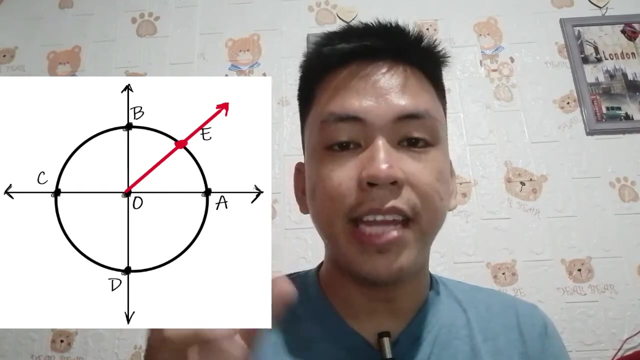 ray. let's say zero e, wherein e is the point in between the points a and b, so zero e. so that may means that zero e forms an angle together with zero a, so that is um a smaller angle compared to zero a and zero b. so that means that is since: